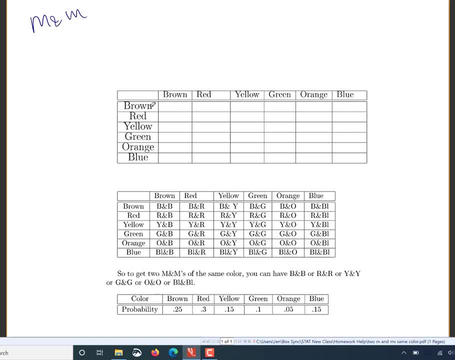 green, orange or blue, And then we're going to look at the intersections here. So if I drew out a brown and a brown M&M, all right here, brown and brown. Or I might draw a brown one first and then red, So that would be brown and red, Or I might draw brown first and then yellow. Let's do brown and. 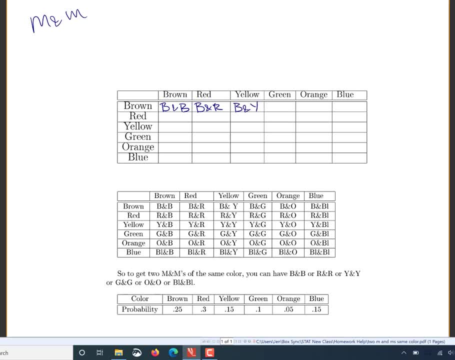 yellow. If I keep going like right here, I can do red and brown, So red and brown. So you'll see there's a lot of different combinations I can get if I draw out two M&M's and look at their color And it turns out so if you come down here, I went ahead and mapped out all of the possible choices. 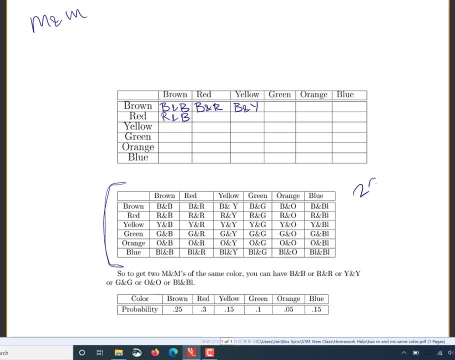 at the same time And you'll notice there are 25 possible combinations Or possible color pairs. We'll call it that. Now. remember our problem said: what's the chances of getting two M&M's that are the same color? Well, let's look on here to find pairs that have. 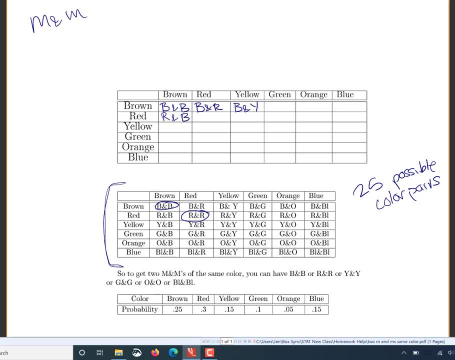 the same color, So I can get brown and brown, Or I can get red and red, Or I can get yellow and yellow, Or green and green, Or orange and orange, Or blue and blue. Now I'm saying or here, because doing blue and blue would satisfy my having two colors. 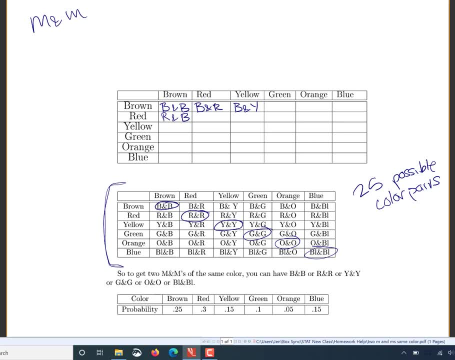 Or I could do red and red, and that would also satisfy what I want. Or I can do yellow and yellow, and that would both be the same pair. So when I'm going through I'm saying, well, this has to be brown and brown, Or I can get red and red. 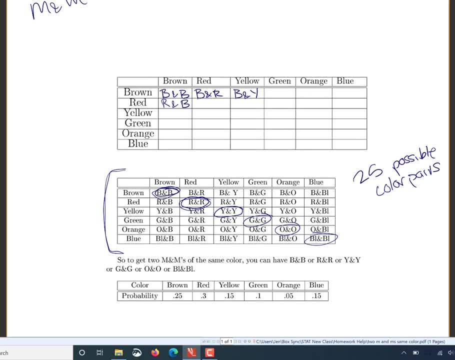 I'm being very particular about what words I use here. So to get two M&M's of the same color, I can have brown and brown, Or I can get red and red- Now red and red is matched together- Or I can get blue and black. Can I have two of the same colors? Can I get two of the? 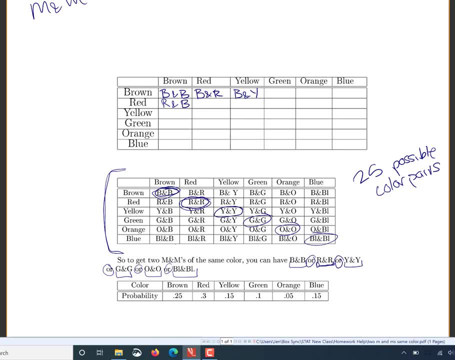 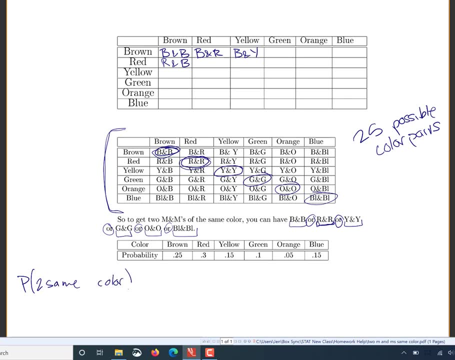 same blue and blue. Can I have two different colors? I can get a color- Cambria. Can I get red and red? Can I get blue and pink, Whether it's the same color? or I can get orange and orange. Can I get blue and blue, Whether it's the same color? so now to 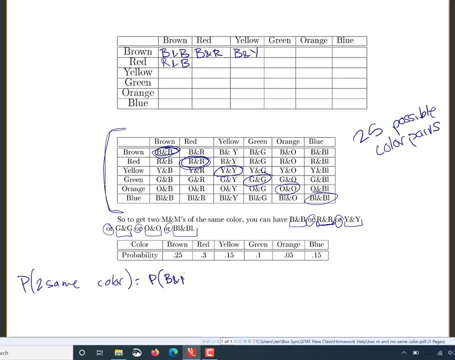 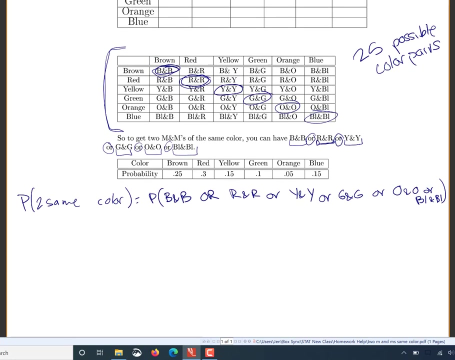 find the probability interviews doing upper half of the patternauen example put in yellow. If you can't see yellow, you let the front back again, Wasn't it before? you can't tell if you're looking for 2 of or orange and orange, or blue and blue. now, anytime you're doing probability, you